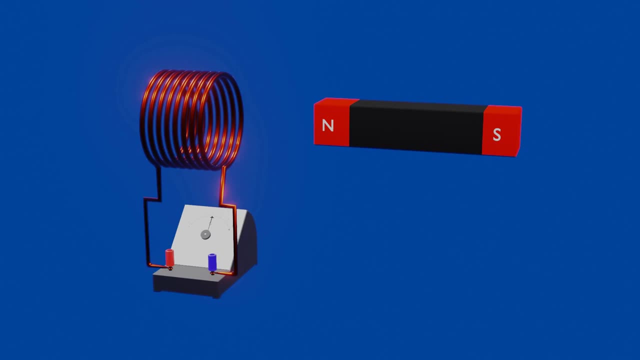 N and S represents north and south pole of a bar magnet respectively. In this bar magnet, N and S represent north and south pole of a bar magnet respectively. In this bar magnet, N and S represent north and south pole of a bar magnet respectively. 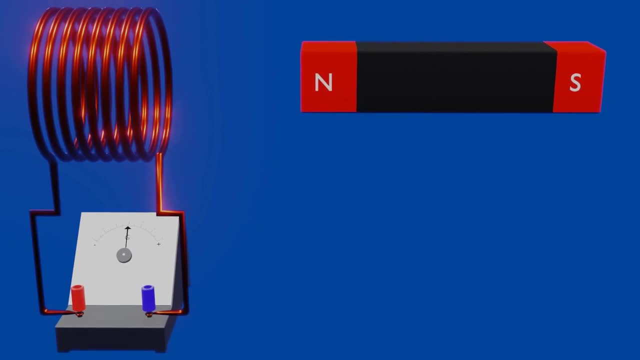 In this experiment. when we move bar magnet towards the coil, then indication of electric current can be seen clearly through the deflection of needle in the galvanometer. But when we stop moving bar magnet, then galvanometer does not show the indication of an electric current. Similarly, when we move bar magnet, 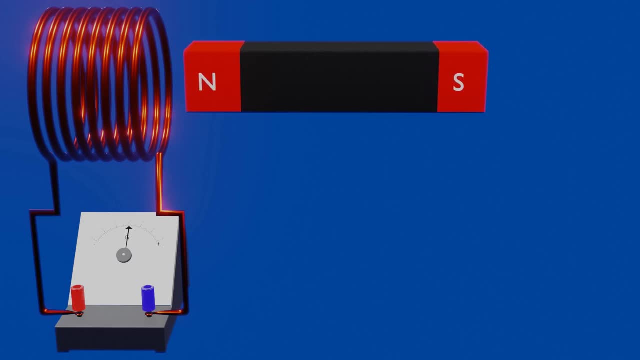 away from the coil. same phenomenon occurs As we are moving the bar magnet away from the coil. there is an indication of electric current in the coil which can be seen by the needle of a galvanometer, But this time needle deflected in opposite direction. and when stop moving bar. 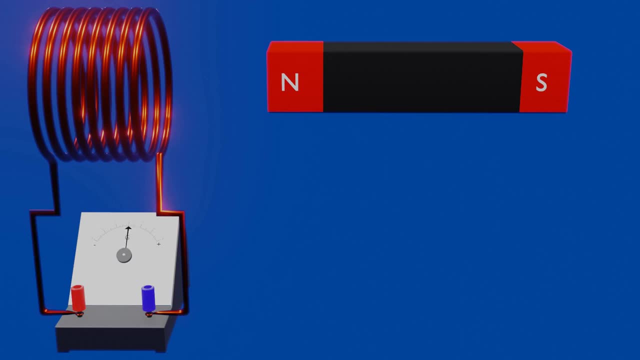 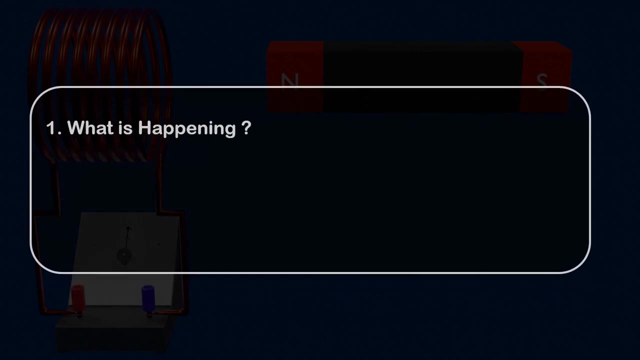 magnet, there is not any indication of an electric current. Now the question arises: what is happening? What causes the charges to flow in the coil? Is it because of motion of the magnet? So the answer is no, But how? Let's explore it. 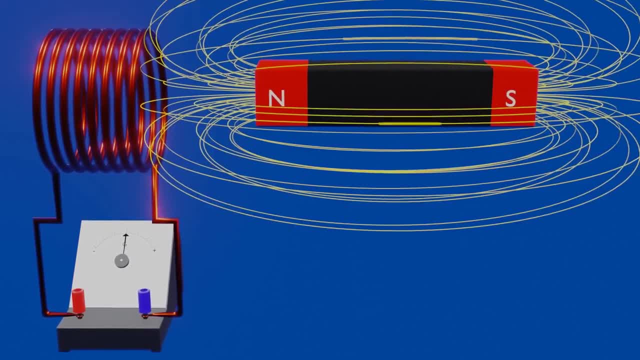 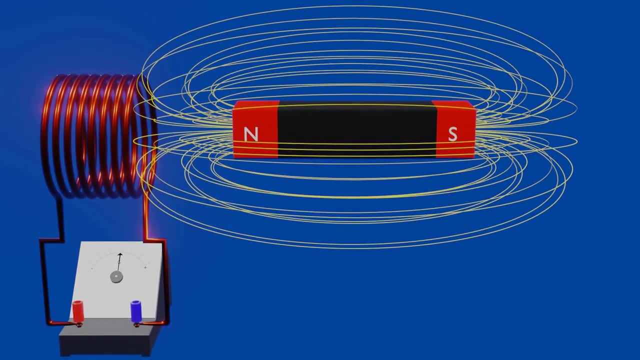 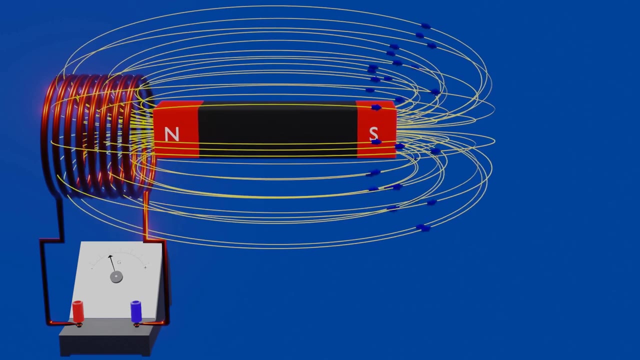 As we all know, bar magnet consists of magnetic field lines emerging from north pole and entering in the south pole of a bar magnet. Therefore, when we move bar magnet towards the coil, magnetic field lines linking to the cross section of the coil increases. 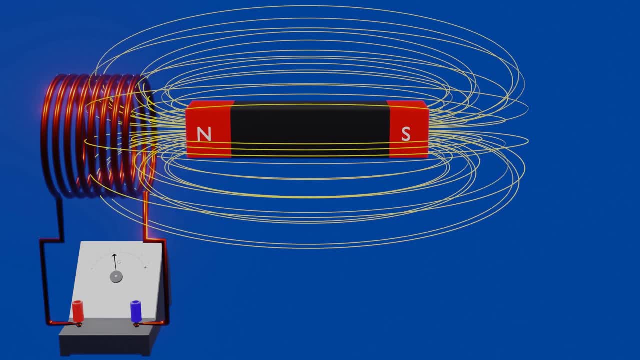 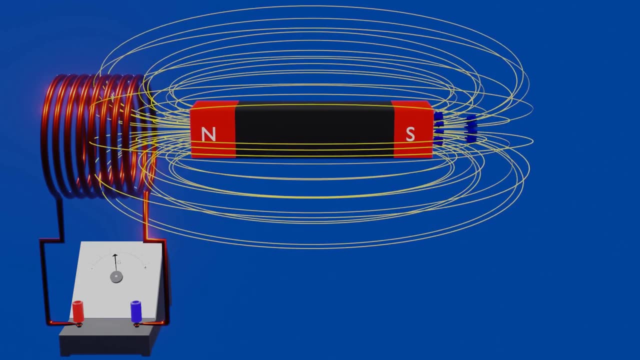 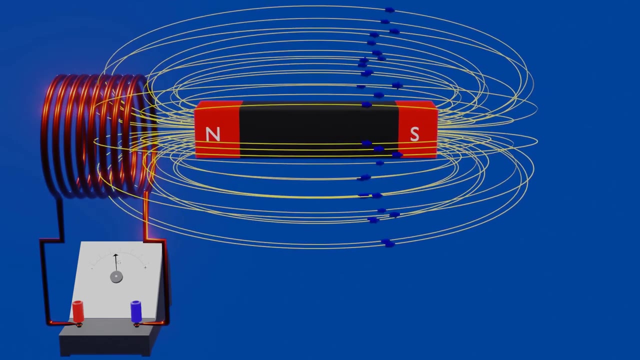 Or we can say that magnetic flux linking to the coil increases as magnet goes nearer to the coil Because of that change in magnetic flux, that is, change in number of magnetic field lines passing through the cross section of the coil, which induces EMF in the coil. 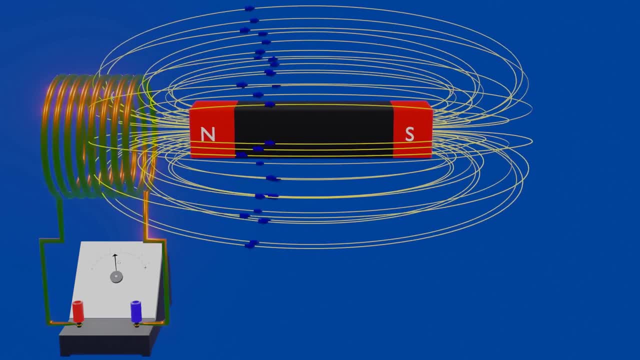 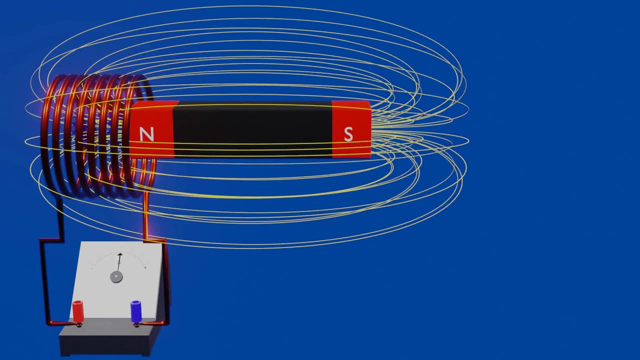 As a result, electric current induces in the coil only if circuit is closed. But as we stops moving magnet, there is not any indication of electric current in the galvanometer. Similarly, when we start moving bar magnet away from the coil, this time magnetic field. 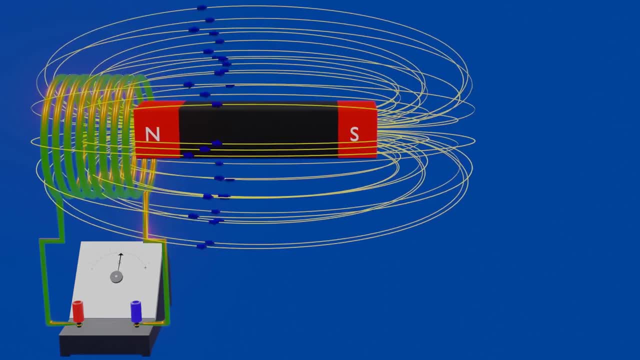 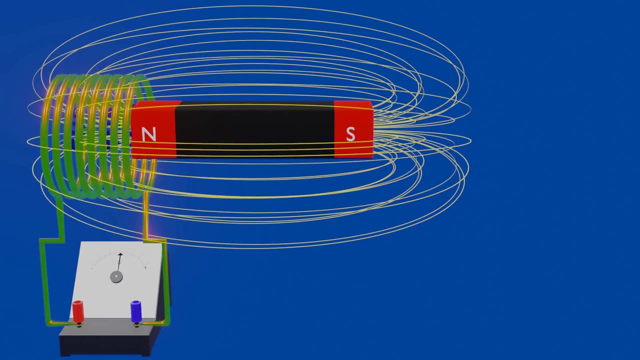 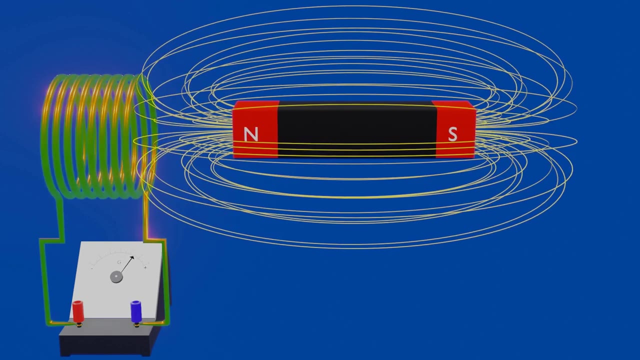 lines linking to a coil decreases or magnetic flux changes. Again, there is indication of electric current as long as we are moving bar magnet away from the coil. It's interesting to note that this time also, induction of electric current stops as bar magnet stops moving. 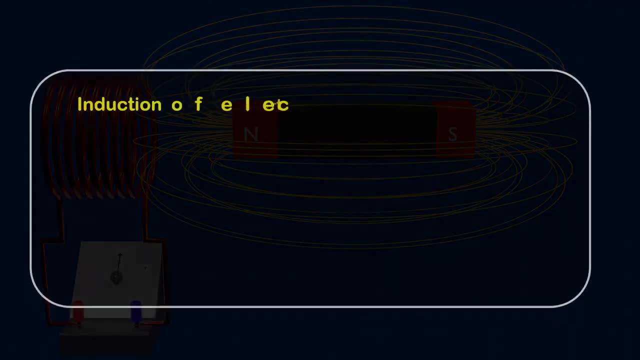 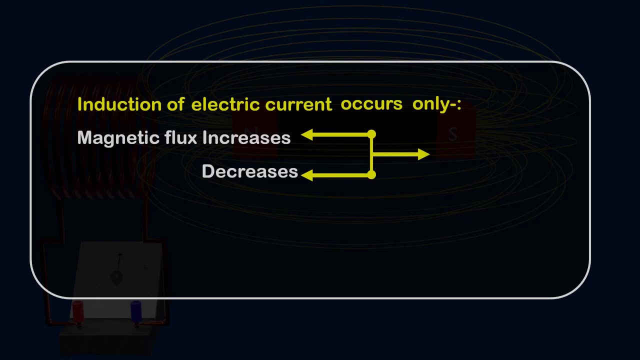 Here it is important to understand that induction of electric current occurs only when magnetic flux increases or decreases, or we can say that there should have to be change of magnetic flux, That is, change in number of magnetic field lines passing through the cross section of the coil. 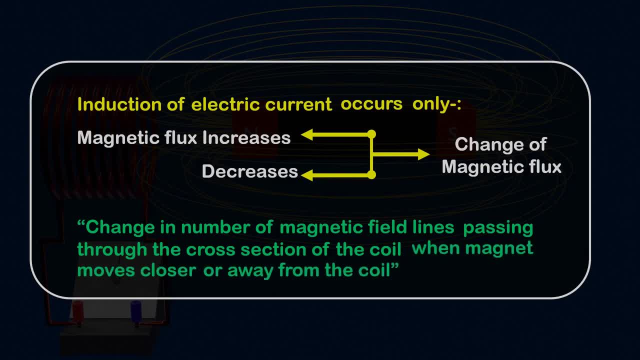 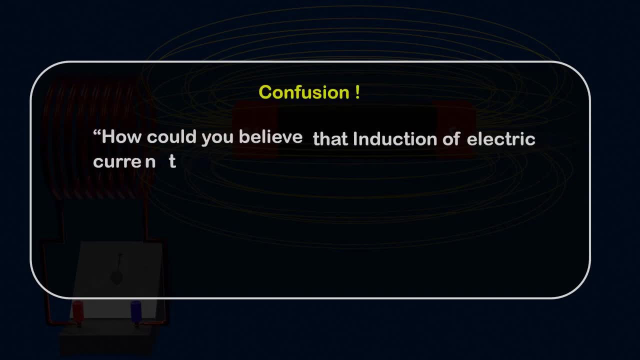 When magnet moves closer or away from the coil. It might have left you with the confusion that how could you believe that induction of electric current is because of change in magnetic flux and not because of motion of a magnet? To make it clear, let's do another experiment. 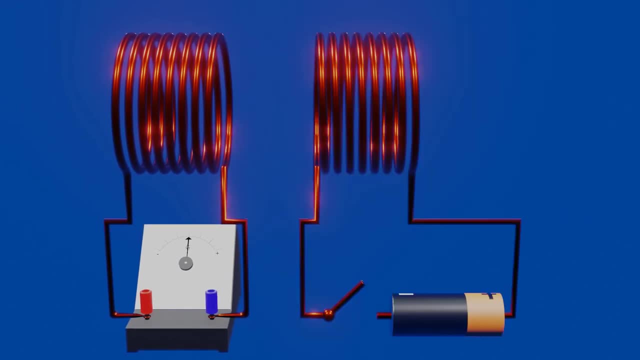 This time we will replace the magnet with another coil which is connected in series with the battery in an open circuit. When we closes the circuit, then just for that moment, the galvanometer, which is connected to the adjacent coil, shows indication of the induced current. 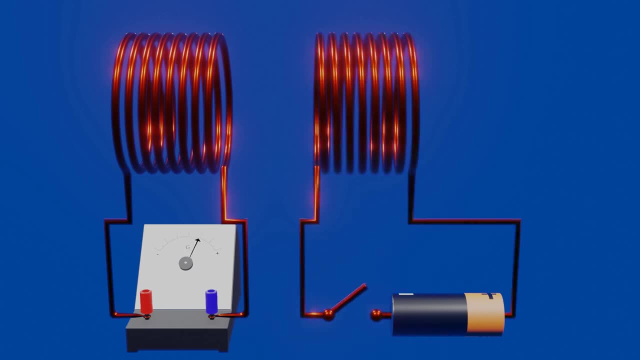 Similar phenomenon occurs when we again opens the circuit, But this time we don't have any magnet or motion of magnet. Then what's the cause of that instantaneous current which only induces for the moment when circuit closes or opens? Let's visualize this: When we closes the circuit, electric current takes some time to reach its highest value. 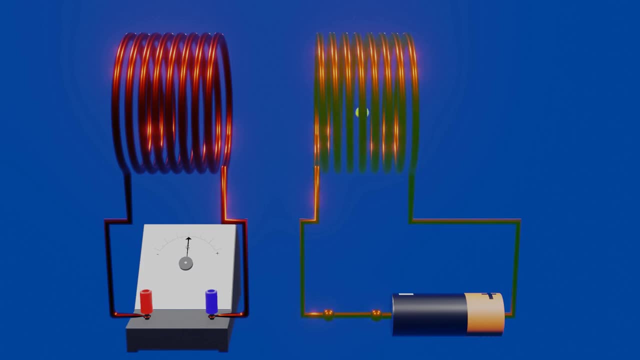 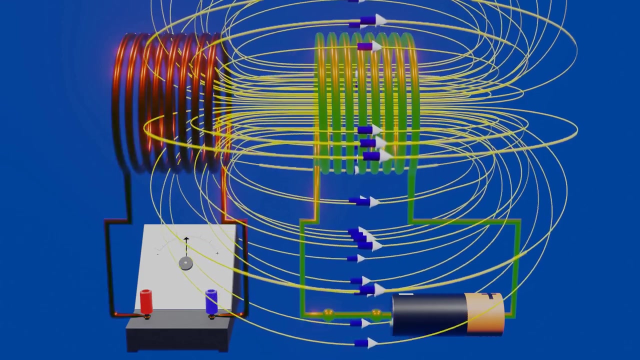 Because of the electromagnetism, coil also starts acting like a bar magnet. Thus magnetic field of a coil also changes from zero to its highest value, in a way that magnetic field lines of a coil starts linking to the cross section of the adjacent coil. 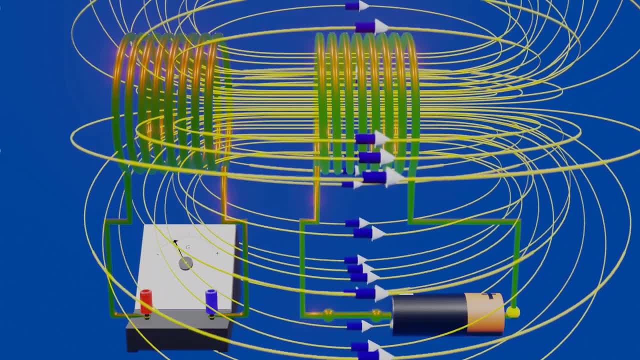 Thus the change in magnetic field of a coil changes from zero to its highest value in a way that magnetic field lines of a coil starts linking to the cross section of the adjacent coil. Thus the change of magnetic flux takes place in adjacent coil, which induces the electric 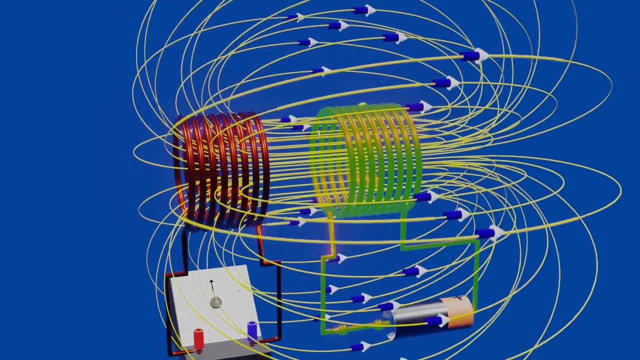 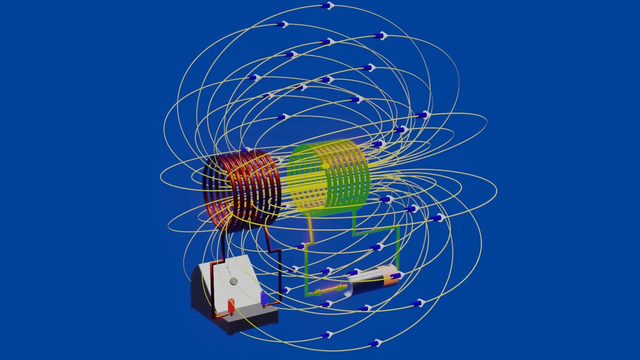 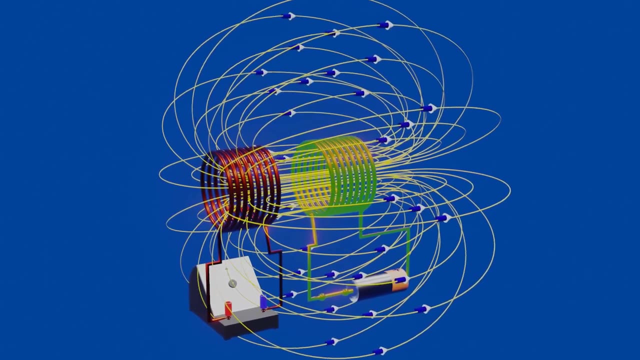 current in the coil for the instant. until current achieves its highest value of producing magnetic field. This change of magnetic flux takes place in very short period of time. So now it's clear that the electric current induces in a coil due to change in magnetic flux, not because of motion of the magnet. 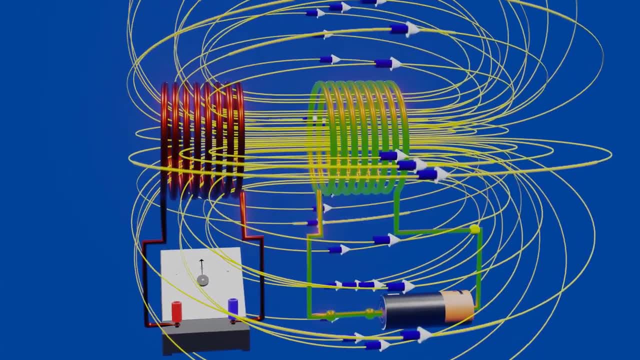 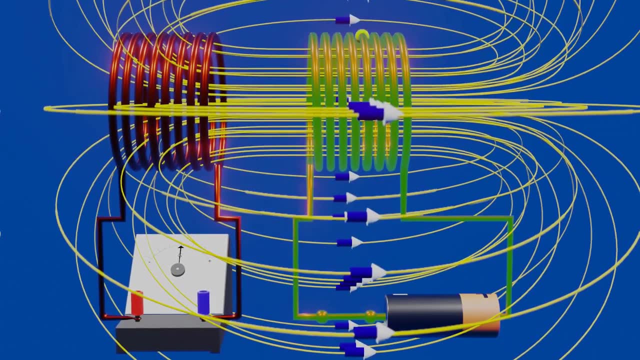 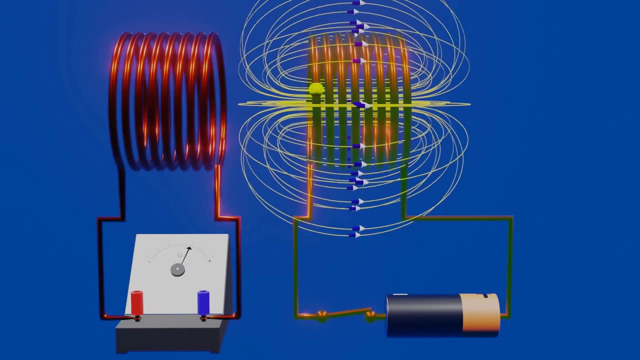 As in this case, There is not any motion involved, But still EMF induced in the adjacent coil which is connected in series with the galvanometer. Similar thing happens when circuit is opened And indication of electric current can be seen clearly in the galvanometer. 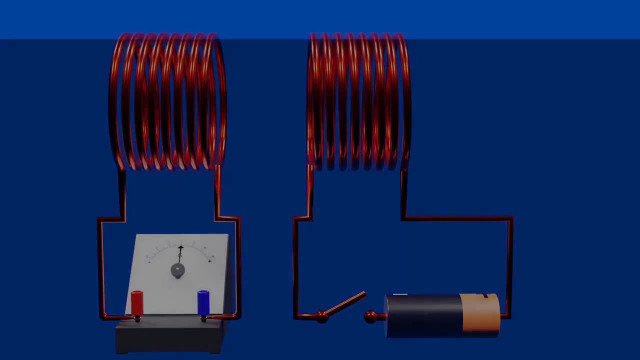 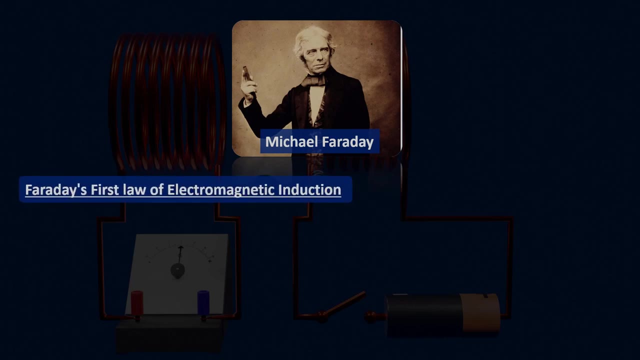 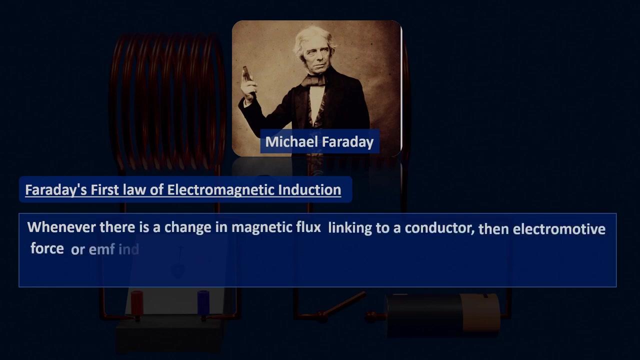 This phenomenon of electromagnetic induction was first experienced by Michael Faraday and named as Faraday's first law of electromagnetic induction. That is, whenever there is a change in magnetic flux linking to a conductor, then electromotive force, or EMF, induces in a conductor, And if the circuit is closed, then this EMF produces current in the conductor. 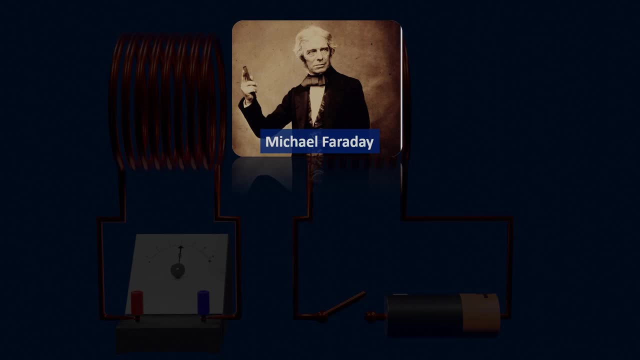 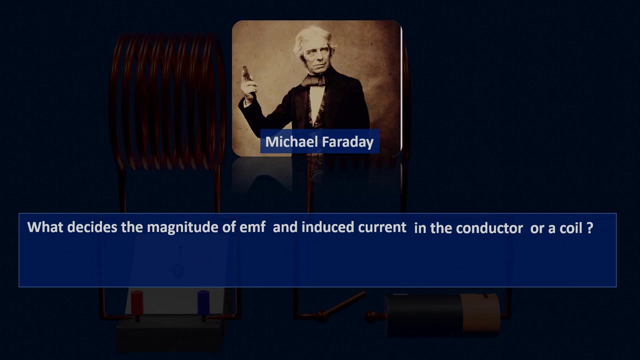 But Faraday's first law of electromagnetic induction only talks about the induced EMF and current, But it does not explains that what decides the magnitude of EMF and induced current in a conductor? Therefore, to answer this question, Faraday given second law of electromagnetic induction, 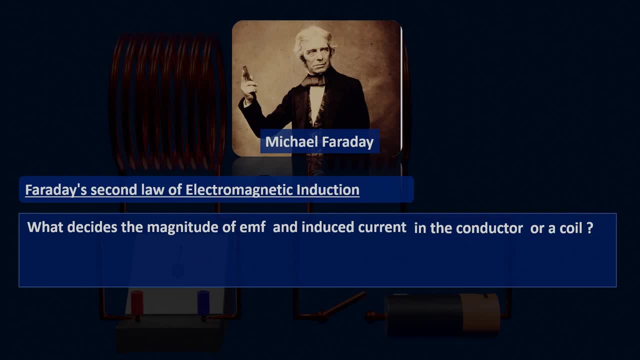 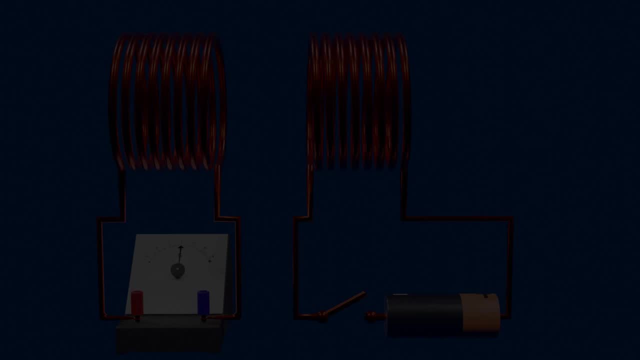 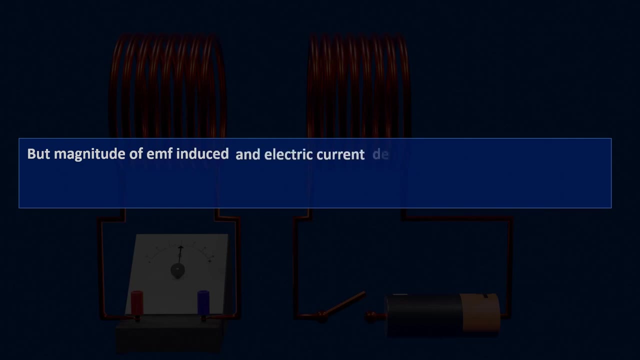 So now let's try to understand Faraday's second law of electromagnetic induction. Now it's clear that change of magnetic flux induces current in the conductor, But magnitude of EMF induced and electric current depends upon the fact that how faster the magnetic flux, that is, number of magnetic field lines passing through the cross section. 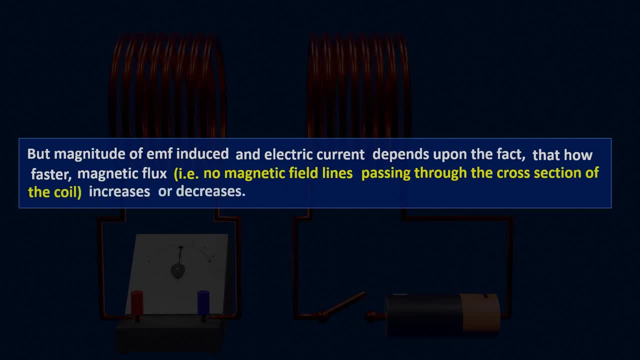 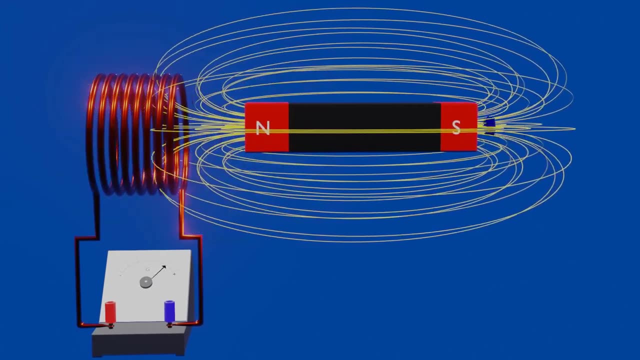 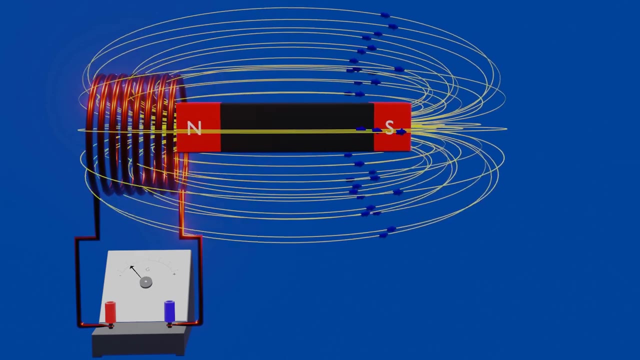 of the coil increases or decreases If we repeat the first experiment, but this time we will move magnet more rapidly, which induces EMF, and then current of higher magnitude will in the coil, which can be seen by the needle of a galvanometer. Now let's try to understand it with the help of magnetic flux. 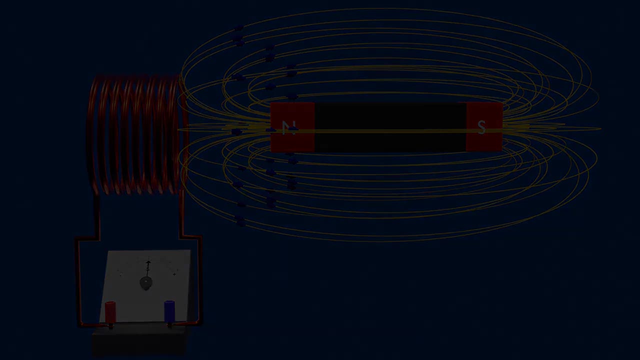 Now let's try to understand it with the help of magnetic flux, which induces EMF, and then current of higher magnitude will in the coil which can be seen by the needle of a galvanometer. So this is the concept of mathematical expression, that is, magnitude of instantaneous EMF induced.